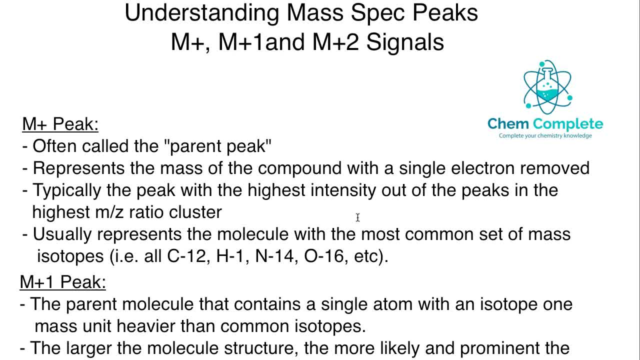 just referring to the mass here. If you take a look at your mass spec and you go up to the area where you see the last grouping of peaks, usually the peak that has the highest intensity out of that grouping is going to be the parent peak. Now it doesn't mean it's going to be the tallest peak. 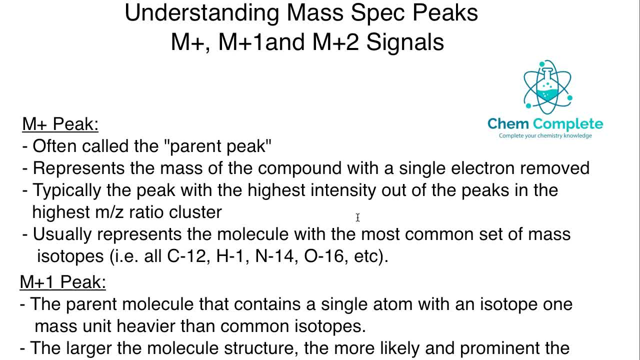 in the entire mass spec. We call that the base peak and we do have a video to help understand the difference between the base peak and the parent peak. I can link that in the description below. Okay, but if you go up to that region where you find the highest set of peaks, the one that is the 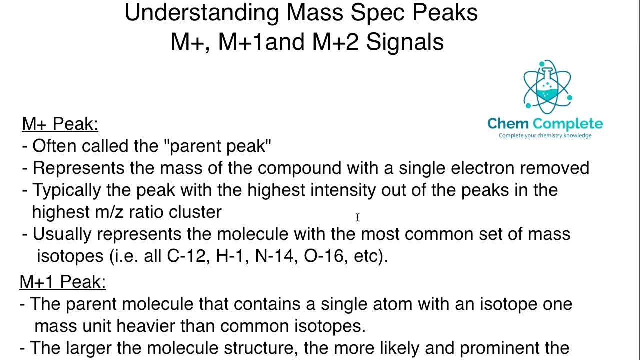 highest out of that group is usually considered the parent peak, which we again refer to as the m plus peak. All right now. usually what this means is this peak will represent your individual molecule and it's going to be a common set of mass isotopes present. So, for instance, if you're dealing with an 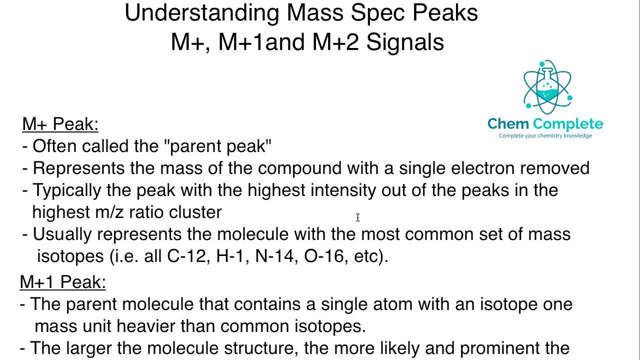 organic compound. it will most likely be dealing with a compound that is completely made out of carbon 12, hydrogen 1, nitrogen 14, oxygen 16.. So, as I'm listing off these isotopes, these are the most common isotopes. For instance, if I have carbons present, there's about a 99 percent chance. 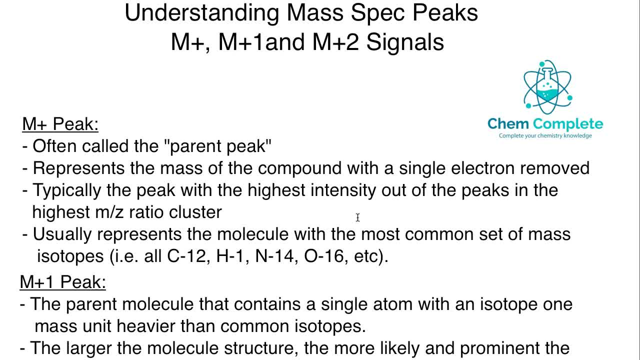 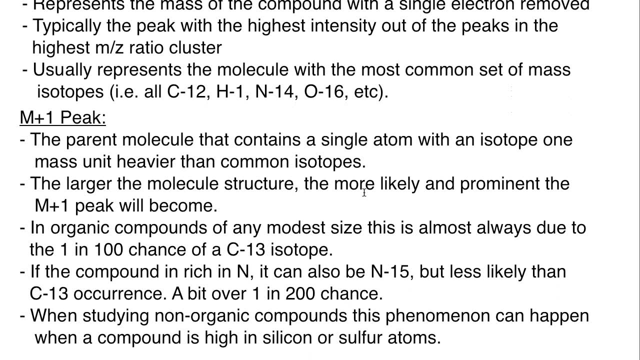 that it's a carbon 12 atom, and so most of the molecules I would expect that I am injecting to this mass spectrometer are going to be made up of carbon 12s. Every 1 in 100 might be a carbon 13, and that leads us into the next topic here, which is the m plus 1 peak. So, keeping in mind that we're 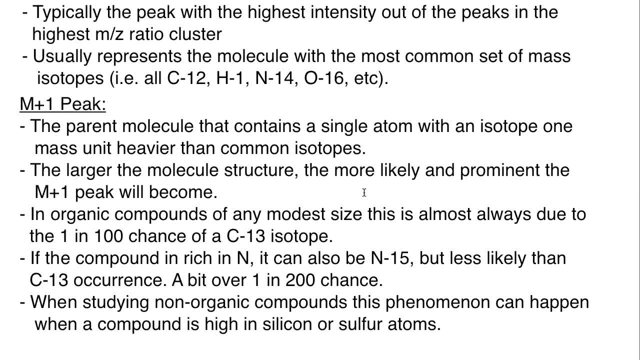 really talking about the mass to charge ratio. when we say m plus 1, it represents the fact that our mass- because the charge is typically going to be 1. when we're using m to z ratio, the mass is simply 1 amu or 1 dalton, whatever you want to call it. So if you're dealing with a mass to charge ratio, 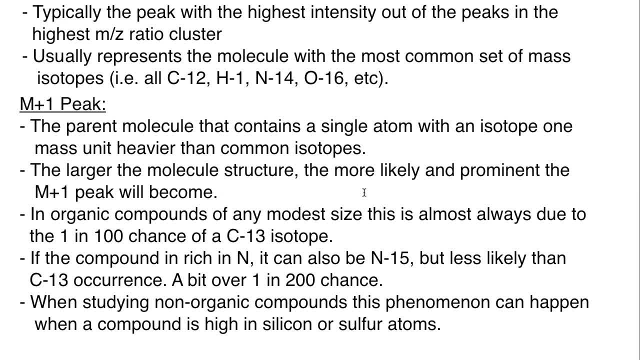 you want to use, it's one atomic unit heavier. So the parent molecule contains a single atom in it that's going to have an isotope with one mass unit heavier than most of the common isotopes. So again, a c13 instead of a c12.. The larger the molecule structure, the more likely this peak is to occur. 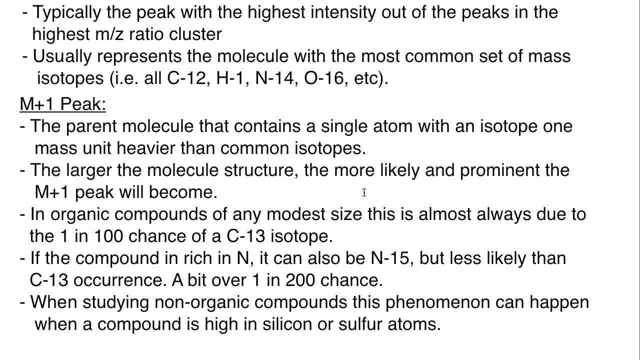 and the more prominent the m plus 1 peak will become. Now, this is nothing but a numbers game when you look at it statistically. So if I have a mass to charge ratio and I have a mass to charge ratio, I have a relatively small organic compound- Let's say it only has five carbons- that I want to 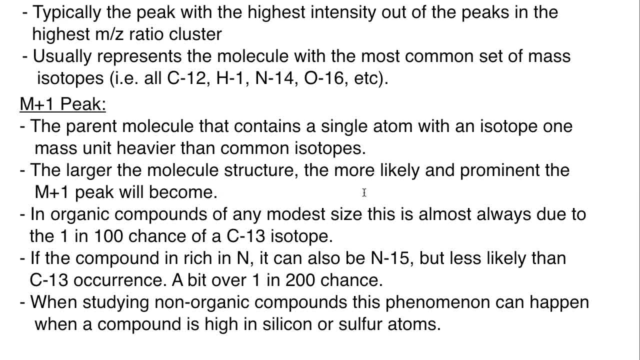 analyze. Well, the chance of finding a carbon 13 is one in a hundred. So there's going to be a pretty small chance that out of those five carbons, one of them is going to be a carbon 13.. But as I increase in size, so let's say that now I'm starting to analyze a compound that has 40 carbons. Well now, 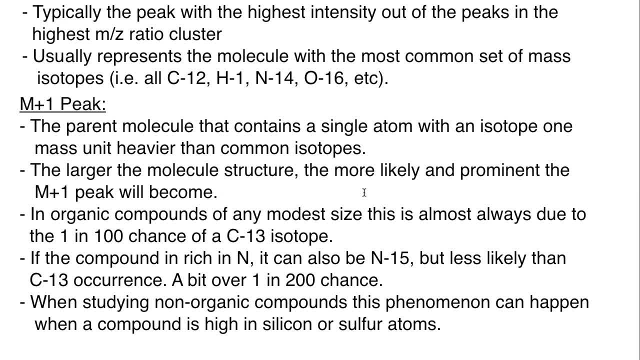 there's a much more higher likelihood, or a greater likelihood, that I could potentially see a c13 in one of those 40 carbons. since the odds are about one in a hundred that a c13 will randomly occur, Okay, so in organic compounds, okay, as long as you have a somewhat modest size, then you will. 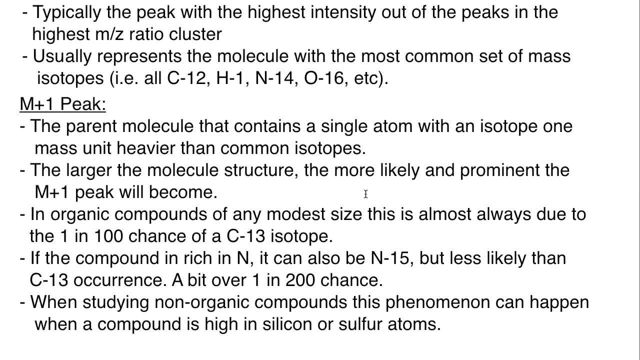 usually see an m plus 1 peak, and that is most commonly due to a c13 isotope. It's about a one in 100 chance. So you can easily see m plus 1 peaks in most organic compounds, provided, I would say, at least somewhere between five to seven carbons. Okay now, nitrogen is another possibility, If you. 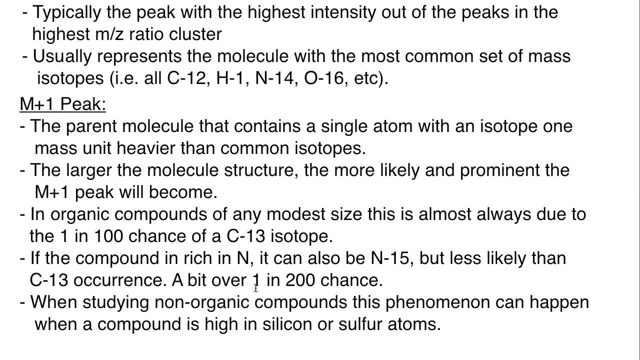 have a compound that is rich in nitrogen- because, remember, organic compounds are going to have far more carbon than nitrogen most often- Okay. but if you do have an organic compound that's relatively rich in nitrogen, you could potentially see a nitrogen 15. that is resulting in an m plus 1. 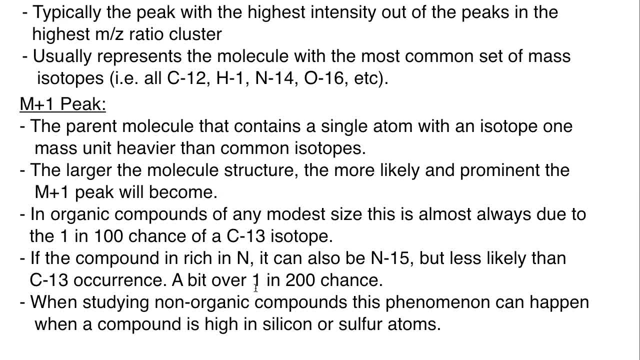 peak, But this is less likely than the c13.. So if you look at the natural abundance, the nitrogen has about a one in two chance. So if you look at the natural abundance, the nitrogen has about a one in two chance. So if you look at the natural abundance, the nitrogen has about a one in two chance. So if 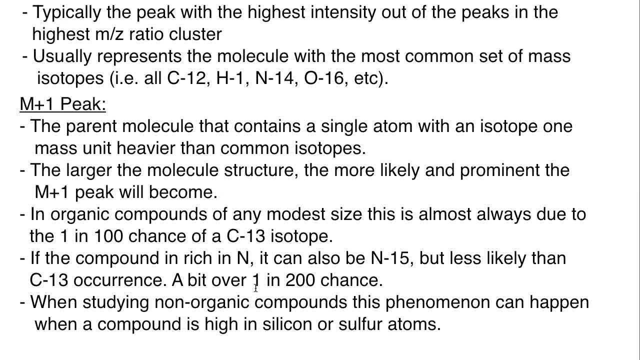 you look at the carbon count, there is definitely a one in two hundred chance of becoming an n15 instead of the one in one hundred chance of the c13. So, again, nitrogen could be responsible for an m plus one peak. but if there's carbon present, especially if there's more carbon than there, 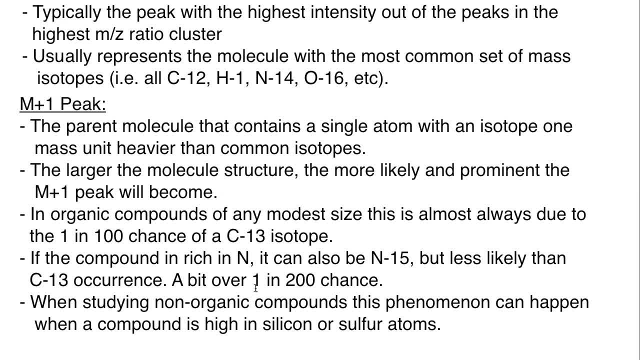 is nitrogen most of the time. the m plus 1 peak is going to be due to the fact that there's carbon 13 present. Now if you are studying non-organic compounds, or potentially if you've got a weird organic compound that has a wholly 100% carbon frenzy presence, it's probably going to be possible. 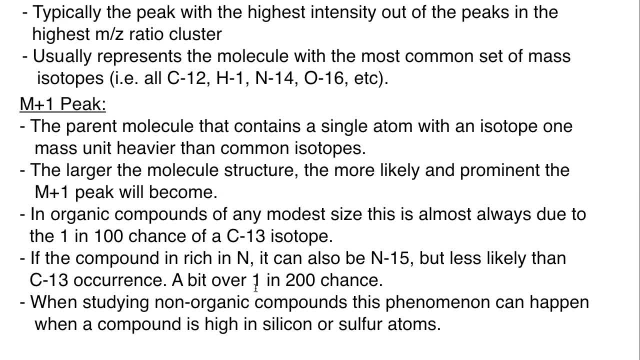 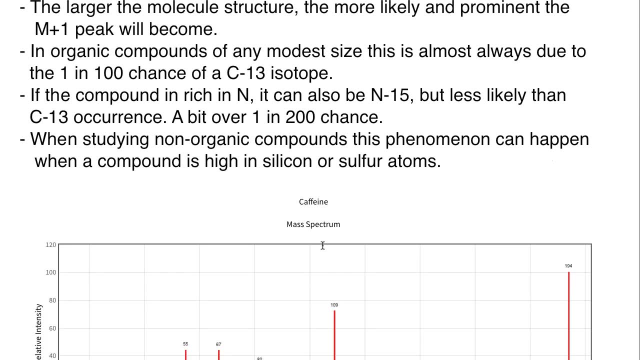 whole lot of either silicon or sulfur, then you may also see an M plus 1 peak. In fact, silicon, if I am not mistaken, has about a 1 in 20 chance. It's about a 4% for the M plus 1 isotope of silicon. Okay, so let's take a look here before we go. 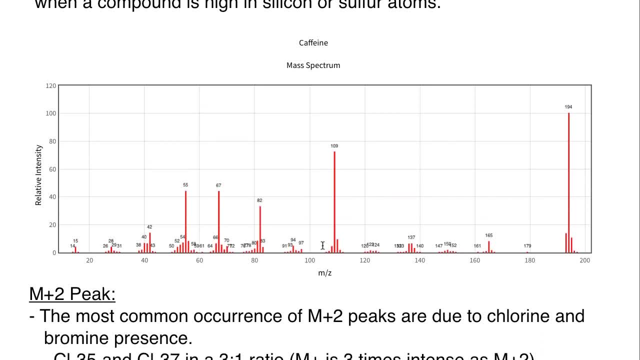 to M plus 2.. We have caffeine. this is the mass spectra for caffeine, and what I want you to notice here is if we come over the grouping of peaks right here are considered to be the highest group of peaks as far as the M to Z ratio is. 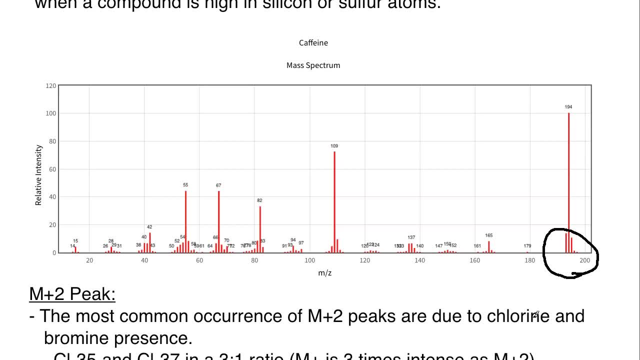 concerned. So of that grouping we can see one of them is far taller, as far as the relative intensity is concerned, than the others, and that is this one right here. This is the M plus peak at 194, so that's the M plus for caffeine. And then, if you 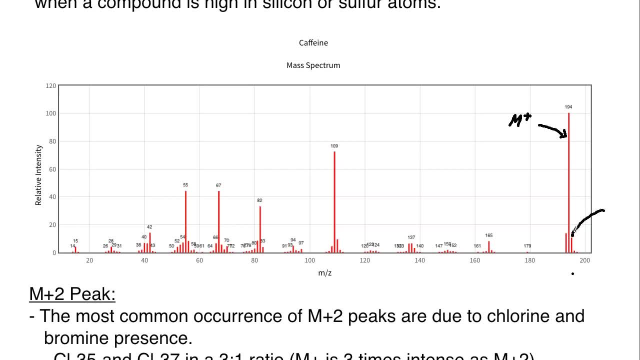 take a look, it's pretty easy to see this here. We have a peak right here next to it. Now it's not labeled as 195, but that's what it would be, and this would be the M plus 1 peak, And then you can also have the M plus 2, and that is. 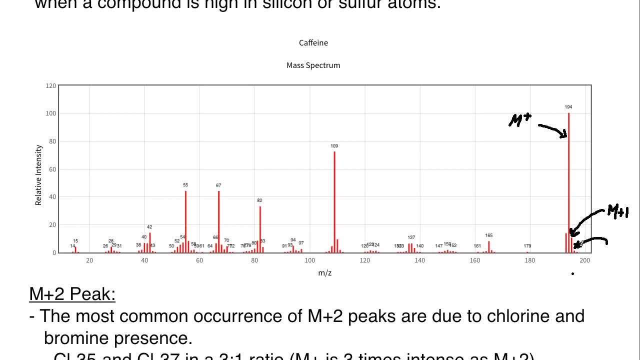 there. It's very tiny relative to the M plus 1, and we'll see why in a minute. Okay, it particularly has to do with, as you continue to go up the ranks like that, there's less and less chance that you're going to see these types of peaks. 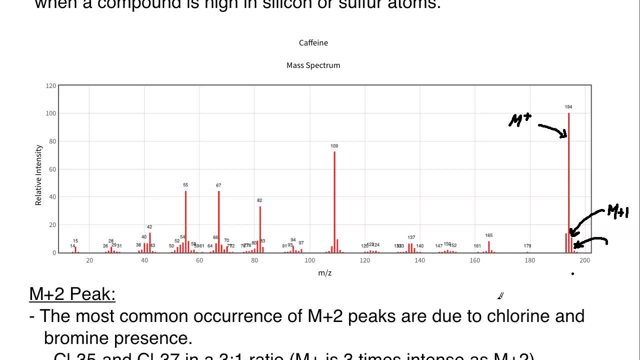 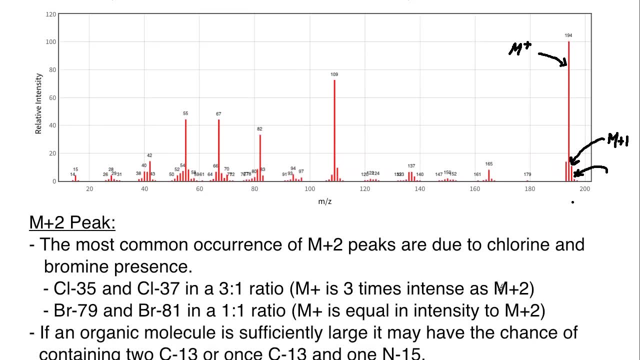 Now that could be due to two carbon-13s, although it's less likely. you'd have to have a whole lot of them. Okay, it's probably due to oxygen, because oxygen can give an M plus 2 peak. All right, so the M plus 2 peak, the. 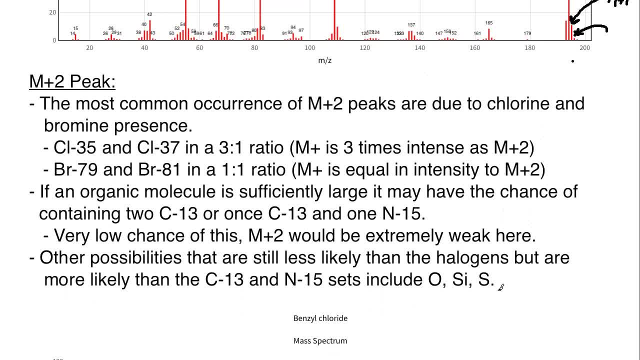 two most common occurrences of M plus 2 by far are due to chlorine and bromine presence in a compound. So these are very obvious, even more so than the M plus 1 carbon-13 peaks. So chlorine has a set of isotopes: chlorine-35 and chlorine-37.. 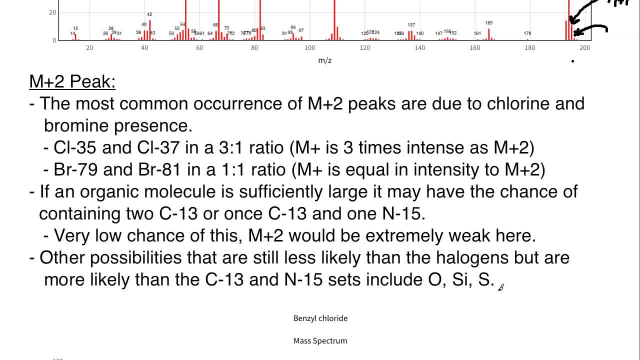 The 35 is the more common one and the 37 is less, so It's about a 75 to 25 percent mix, or a 3 to 1 ratio, All right. so if chlorine is present, the M plus peak is going to be about three times as intense. 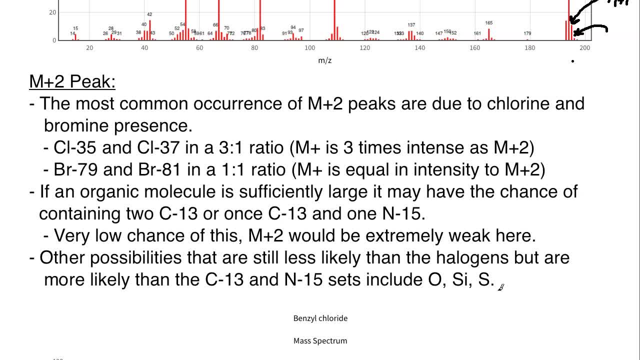 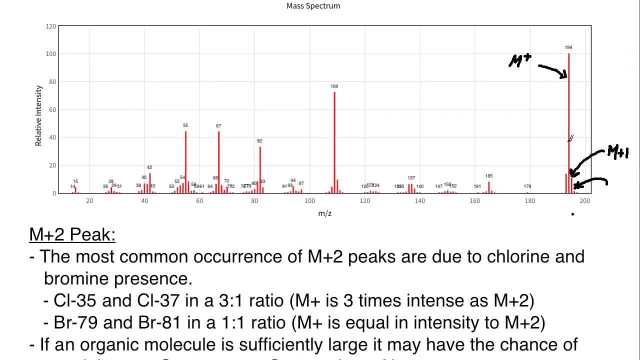 as your M plus 2 peak. So if your M plus 2 peak is about a third the size of your parent peak, go up and look at caffeine. If you had one that was about the third the size of this peak, that's going to be very evident in the M plus 2 spot. You'll 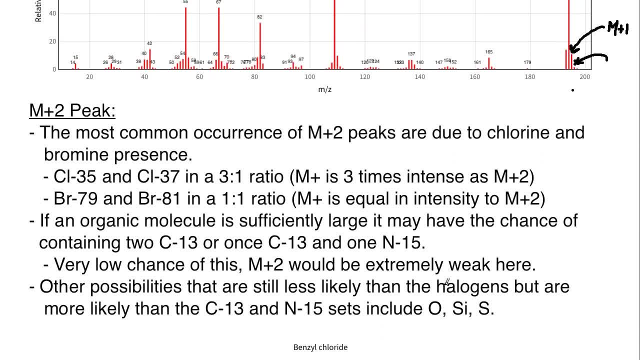 see a pretty large peak there. Okay, now bromine. you have bromine 79 and bromine 81. They are in a one-to-one ratio, relatively speaking, for isotopes, And so you will see an M plus that has an equal intensity peak at M plus 2. They will be almost dead even with one another. 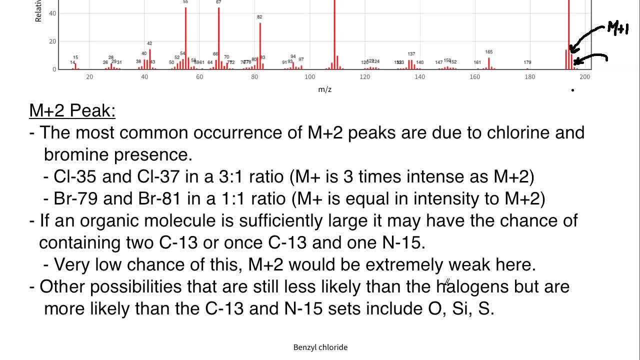 as far as the statistical occurrence of them. Okay, so chlorine and bromine are the two most common sources of M plus 2 peaks, especially ones that are very prominent, that we can easily see. And then we have the M plus 2 peak, which is: 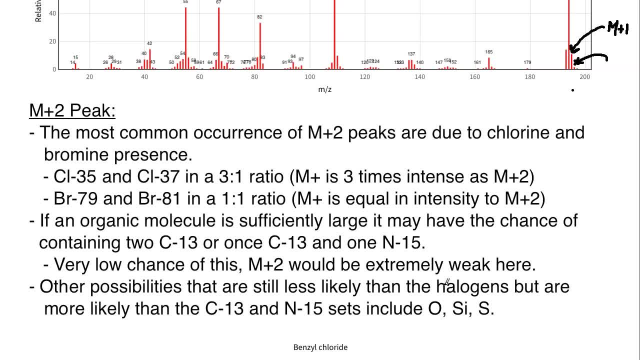 C. Now, if an organic molecule is sufficiently large enough- and it has to be pretty large- in order to pull this off, it could potentially have an M plus two peak due to two carbon 13s in one molecule. Now again, the chance here is one in a hundred. So now you're trying to take. 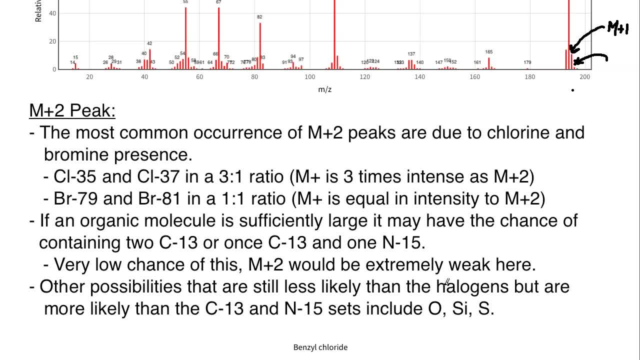 that one in a hundred chance and say it's going to happen twice in the same molecule, You are getting into shaky territory in terms of statistics. It's not that it's impossible, but it starts to become pretty improbable, unless you're going to have a very large organic molecule. 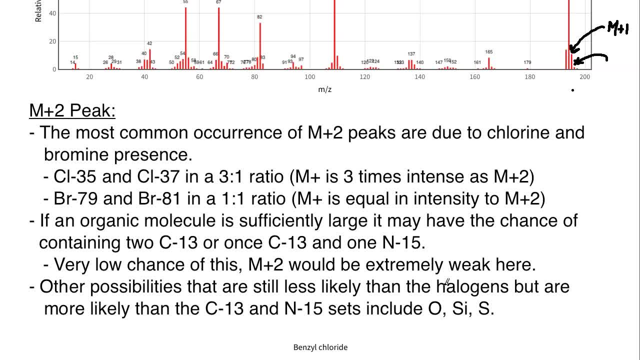 where you've got a whole bunch of carbons, and it's certainly more possible at that point that you could see several C13s that might be present. Okay, same thing for a C13 and a nitrogen 15.. So we could have one carbon 13 and one nitrogen 15. This would be even less likely because nitrogen 15. is less likely to happen. So we could have a C13 and a nitrogen 15.. So we could have one carbon 13 and a nitrogen 15.. So we could have one carbon 13 and a nitrogen 15.. So we could have one carbon.